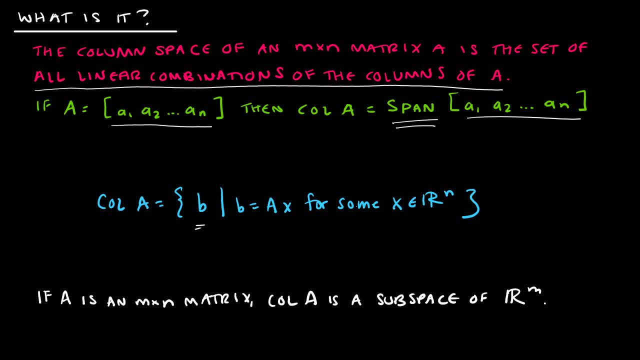 prove that one because we know, based on a proof- I think we proved it in a previous video, either that, or we just talked about it- that the span of vectors is in fact a column space of RM. So we're not going to prove that, but just know- that is a theorem in your text- that the column space of A. 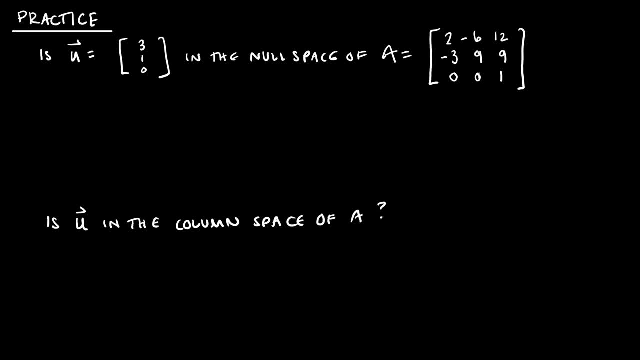 is a subspace of RM. Here's a great practice for us, not only in null space, but also in column space. So we've got one vector A and, I'm sorry, one matrix A and one vector U and I'm asking if U is in the null space and if U is in the column space. So this would be a good practice to help us to know exactly how to go about solving these. So, as a reminder, if we're looking at null space, we're saying that A times U would have to be zero for this to be true. 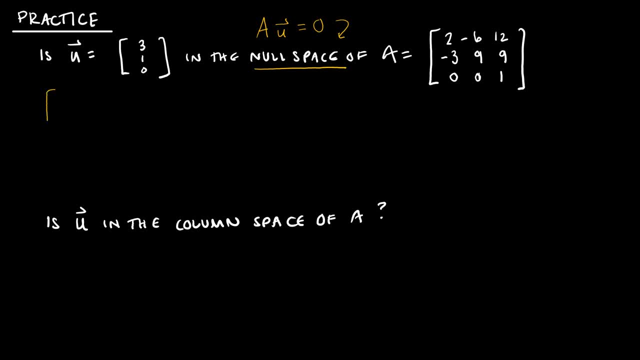 So that's pretty straightforward. all I have to do is do some multiplication: 2, negative 6, 12,. make sure you multiply in the proper order: negative 399,001 multiplied by vector U, which is 310.. That's going to give me. 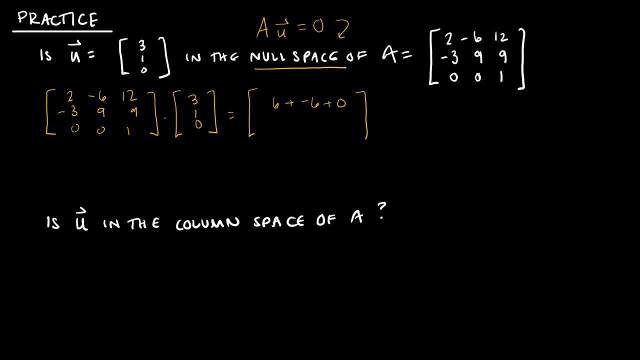 6 plus negative, 6 plus 0, and then negative 9 plus 9 plus 0, and then 0 plus 0 plus 0, and I end up with 0 0 0. and because this is the 0 vector, which is what I was looking for, then I can say: therefore, U belongs to. 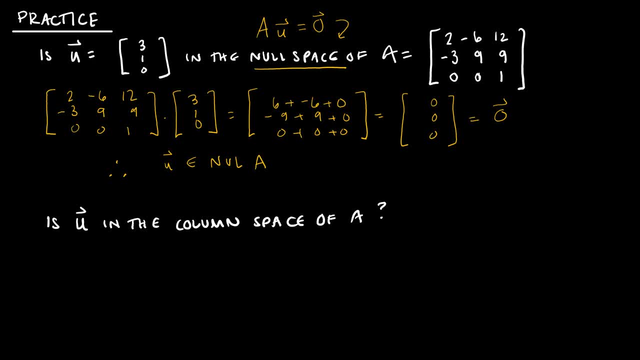 null A. so now let's switch gears and talk about the column space. for the column space we're going to take A and augment it with U and then we're just going to do row reduction and determine if it's a consistent system or inconsistent. so if the system is consistent, then U would be in the column. 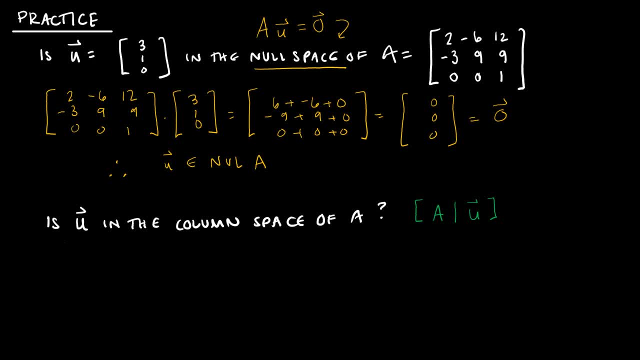 space of A, and if it's inconsistent then it's not. so that means I've got a 2 negative, 6 12 negative, 3, 9, 9, 0, 0, 1 augmented with 3 1 0, and I'm just going. 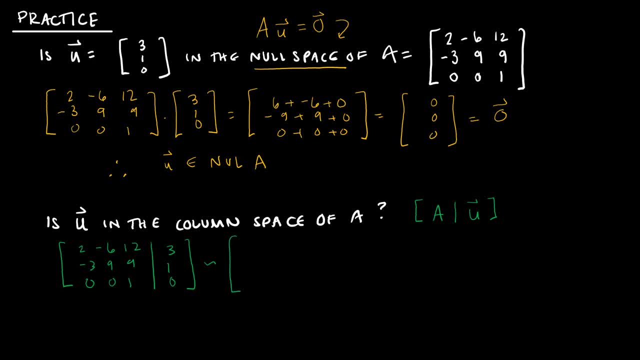 to do my row operations. so again, there's really no right or wrong way to do your row operations. I'm just trying to get it to the point that's either in reduced row echelon form, or I find out that I don't have enough pivots and 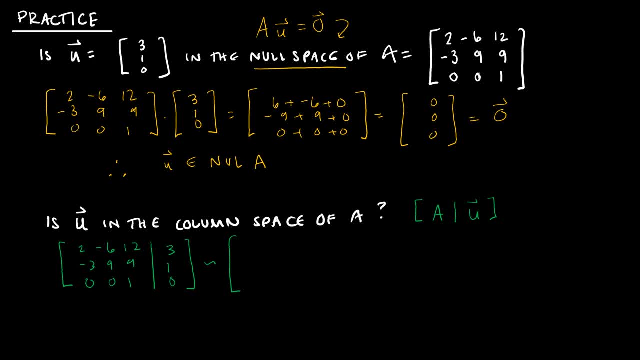 therefore, it's inconsistent. so the first thing I'm going to do is I'm just going to reduce my first row by 1- half- oops, that is not 4, half of 12, still 6- and then I'm going to reduce my second row by negative 1, 3rd. so that gives me. 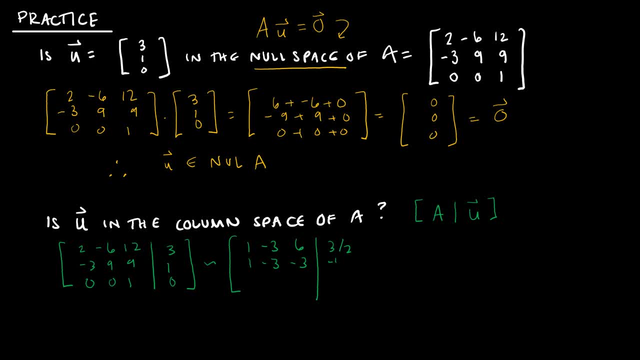 positive, 1 negative, 3 negative, 3 negative, 1 3rd and 0 0, 1 0. so it's pretty clear I'm going to have a pivot here. and it looks pretty clear I'm going to have a pivot here, probably, but let's go ahead and 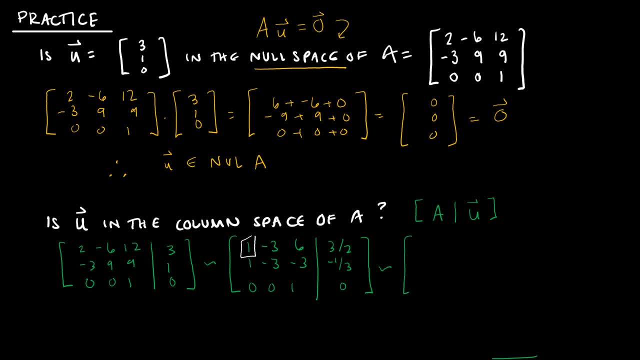 keep going. if I do another row operation, I'm going to keep this 1, 3, 6, 3 halves and then I'm just going to subtract the two rows. so 1 minus 1 is 0 negative. 3 minus negative 3 is 0.. 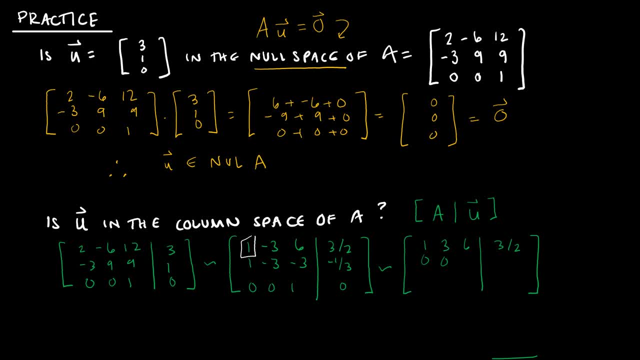 negative 3 minus negative 3 is 0. negative 3 minus negative 3 is 0.. 0,. 6 minus negative 3 is 9, 3 halves minus negative 1. third is 11. sixths, and this is: 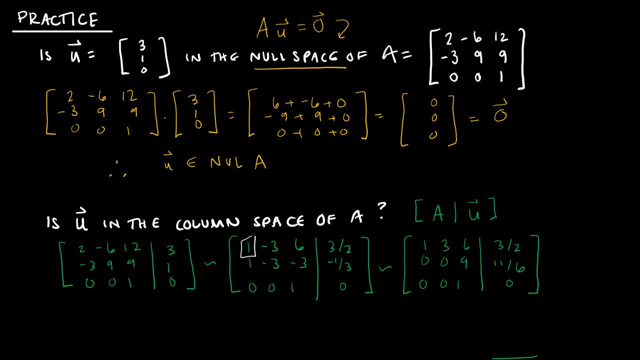 0, 0, 1, 0. And then, hopefully at this point you can see that there is no pivot in the second column and therefore this is inconsistent. You could obviously keep going, and if you kept going you would end up with a 0, 0, 0,. 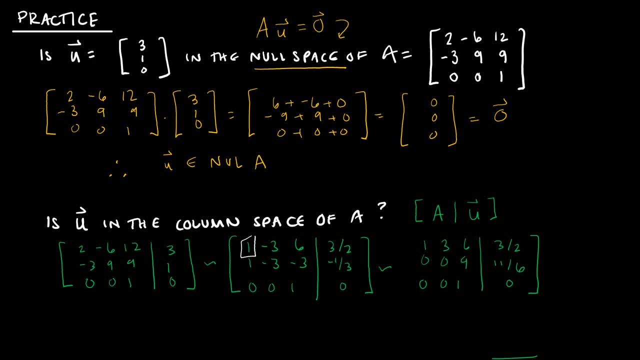 0, but it's really not necessary, because once I got to this point, it's pretty clear that there are not enough pivots. So, because this is inconsistent and then therefore U does not belong to the column space of A, Here's another practice for us to try. 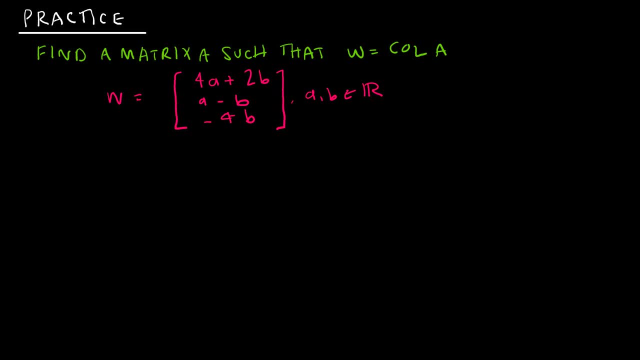 This one asks us to find a matrix A such that W is equal to the column space of A, and then it gives us this matrix W, which is sort of defined in a weird way, But this is actually a fairly straightforward question. I know that W can be rewritten as a linear combination, so I can say that this is A times. 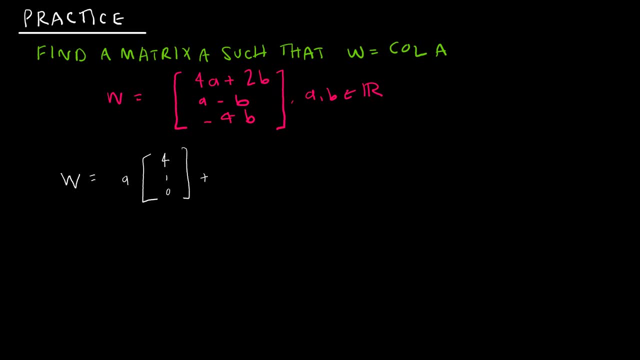 4, 1, 0 plus B, to negative, 1, negative, 4.. And then, of course, A and B are real numbers, And so essentially what I'm saying is: this is the span of 4, 1, 0 to negative, 1, negative. 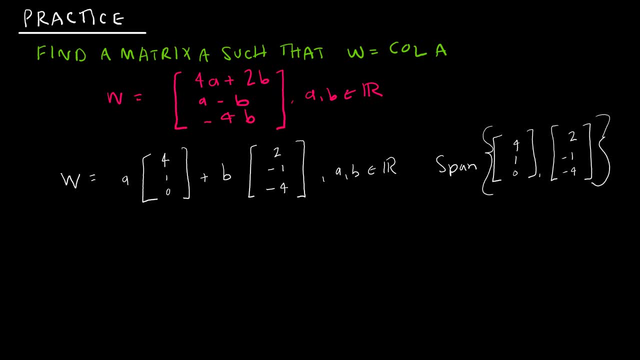 4.. Okay, Awesome, But I still haven't answered the question, because the question says: find a matrix A. So what they want me to do is find a matrix A. Well, no problem. A is then 4, 1, 0, 2, negative, 1, negative 4.. 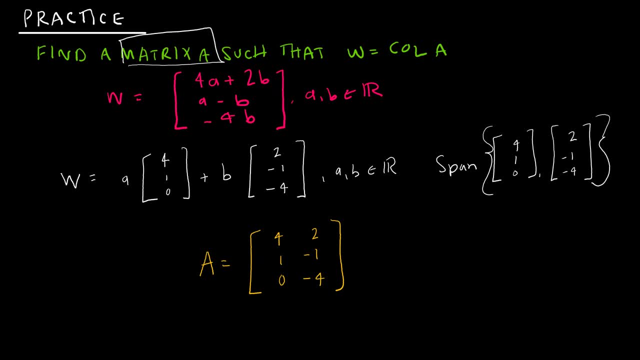 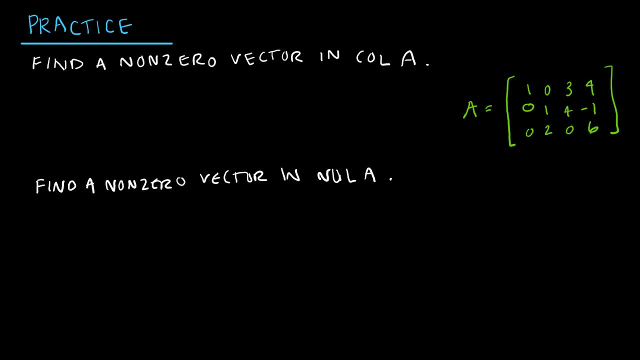 There's my matrix A that exists, such that W is equal to the column space of A. Here's a great practice for you to try on your own. So I would like you to try this one and when you're ready, press play to see how you did. 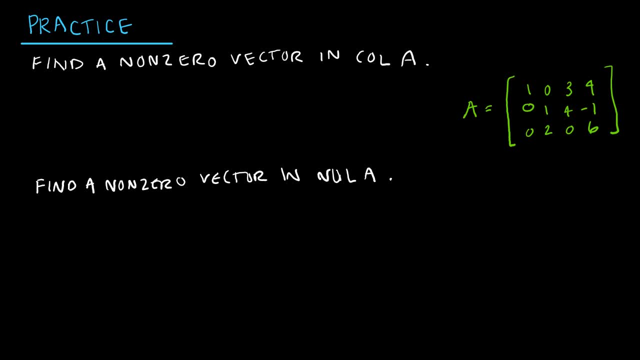 If we're not quite there yet, that's okay, You can just wait and I'll go over it with you. All right, let's take a look. I'm asking you to find both a non-zero vector in the column space of A and then one in the null space of A. 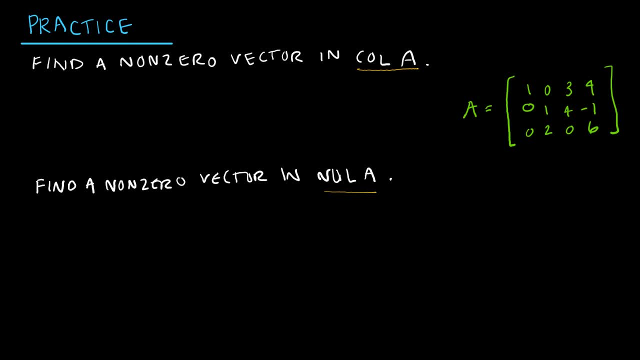 And you'll find that the non-zero vector in the column space of A is any one of these columns written as a vector. So I'm going to choose, say, 4, negative 1, 6.. That is a perfectly good solution. 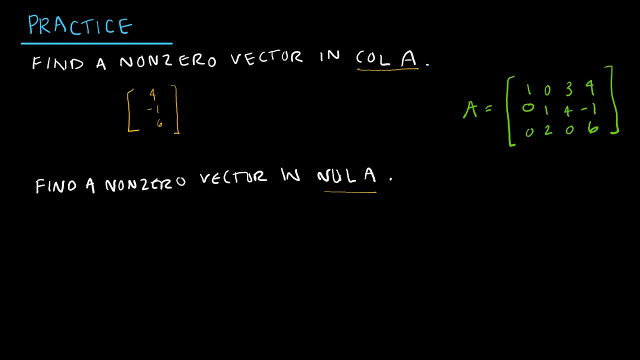 I could have chosen any one of those columns and that would all be the correct solution. For the second part, a non-zero vector in the null space of A requires me to take A and row, reduce it and augment it with the zero vector. 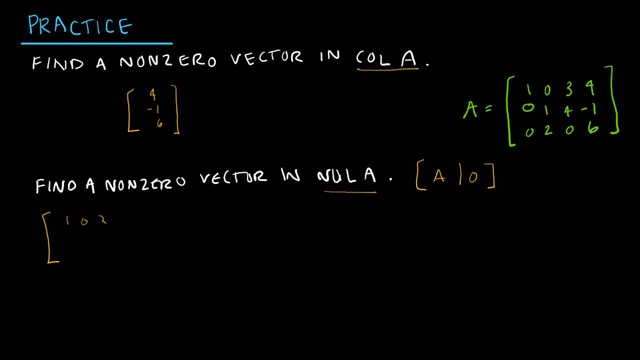 So I'm going to take 1, 0,, 3,, 4. 0, 1, 4, negative 1. 0,, 2,, 0, 6. Augmented with the zero vector And do some row reductions. 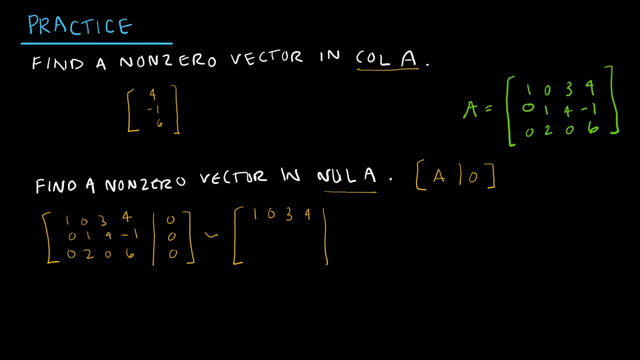 So I like my first row. I've already got a 1, and I've already got a 0.. And I actually like my second row, because I have a 0 and a 1.. So far I've got a pivot and a pivot. 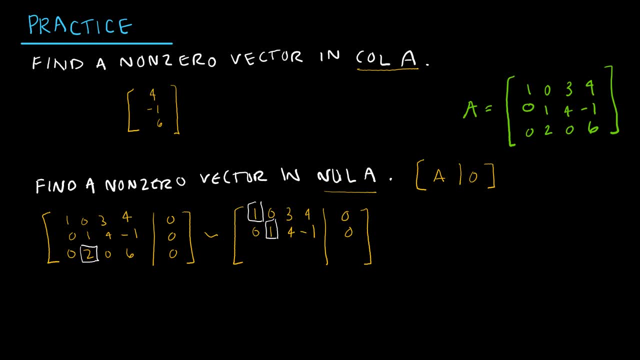 And I need to turn this guy into a 0.. So let's take 2 times row 2 and add it to row 3.. So I get 0.. I'm sorry, subtract row 3.. So 2 times 1 is 2, minus 2 is 0.. 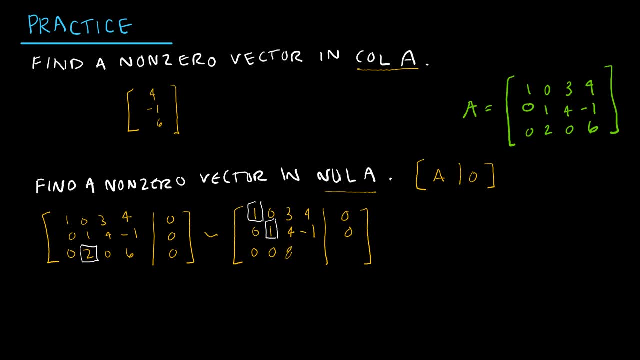 2 times 4 is 8, minus 0 is 8.. 2 times negative: 1 is negative 2, minus 6 is negative 8.. And then, of course, 0.. Continue, Continue, Continue with my row operations. 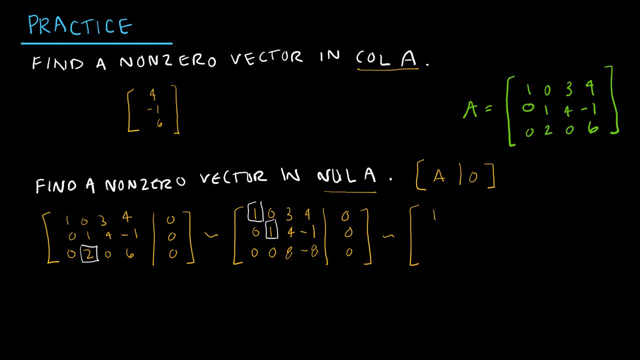 So my first column's great, My second column's great. I'm going to leave the first and second rows exactly as they are for now, And in that last one I'm going to take it times 1- eighth. So that gives me 1 negative 1.. 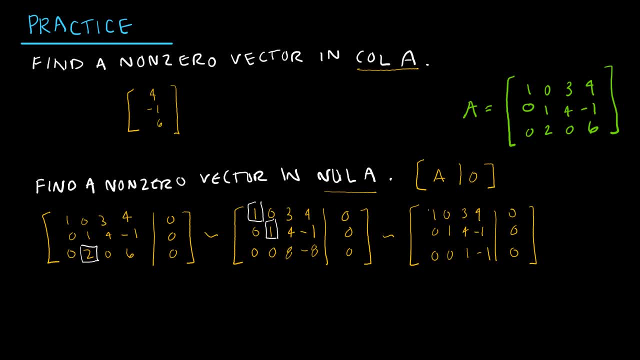 And then I'm almost where I want to be. I've got a pivot, I've got a pivot, I've got a pivot And I've got a pivot. But what I don't have is I need a 0 and a 0.. 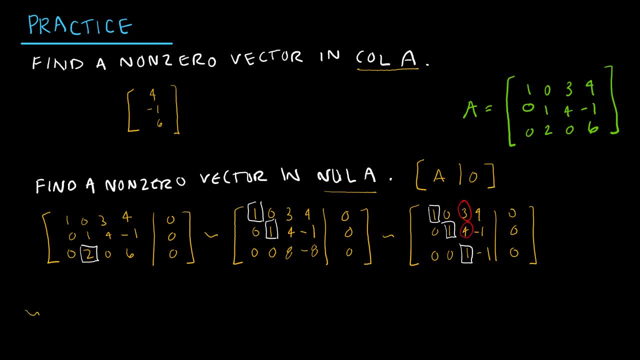 So let's keep going. That's going to give me first row. I'm going to take my third row times negative 3 and add it to my first row, So I get 1, 0, 0.. And then 3 plus 4 is 7, 0.. 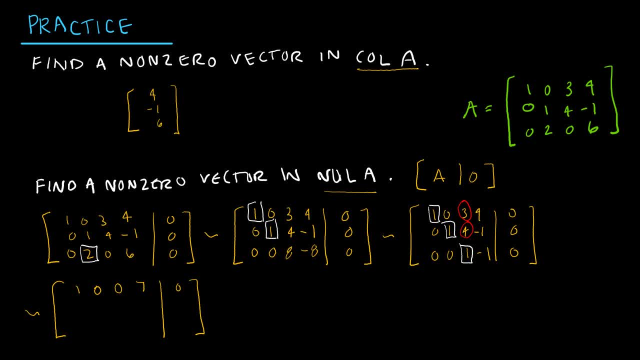 And then for my second row, I'm going to take my third row times negative 4 and add it, So I get 0, 1, 0.. And then that's positive 4 plus negative 1.. So that's positive 3.. 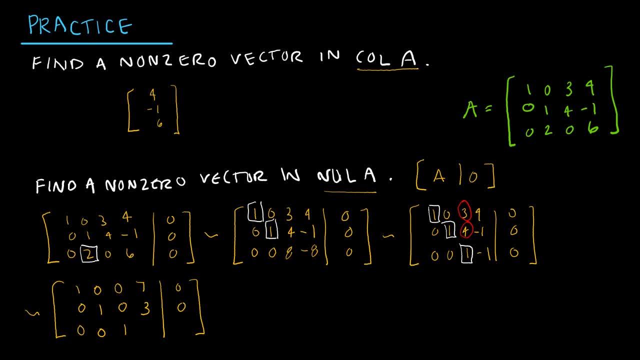 And then this guy I didn't do anything to at all. So what am I going to do from here? Well, I know that my solution is that x1.. x1 is equal to negative 7x4.. And because obviously x4 is my free variable, 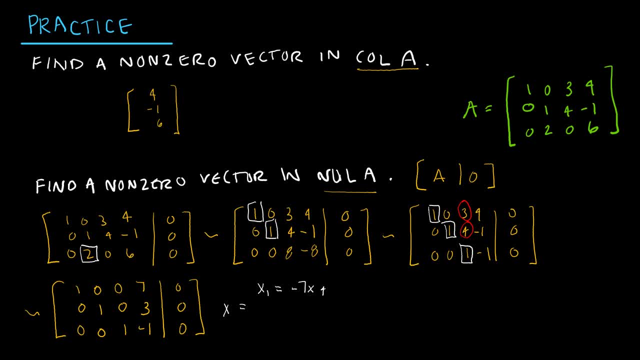 And so that's the only one I should have here. And then x2 is equal to negative 3x4. And x3 is equal to 1x4. And x4 is free. So really my solution here, if you'll recall. 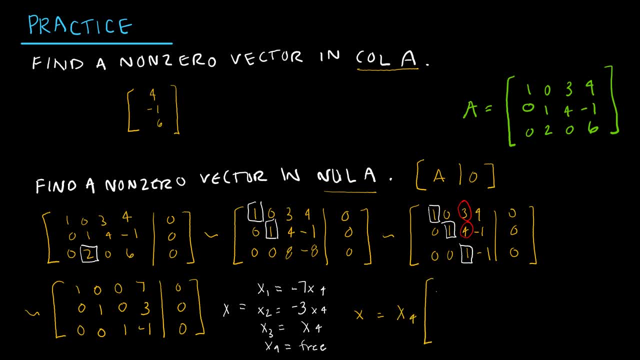 is that I can write it negative 7, negative 3, 1, 1.. And from here I'm looking for again a non-zero vector, And so what that tells me to do is essentially come up with some x4. 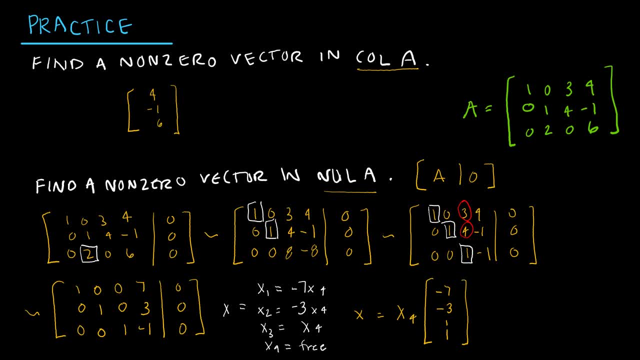 So whatever x4 I want And then multiply it. So let's just say x4 is 2. So a non-zero vector in the norm. And then if I try to find the everyday state, which is the null space of a, 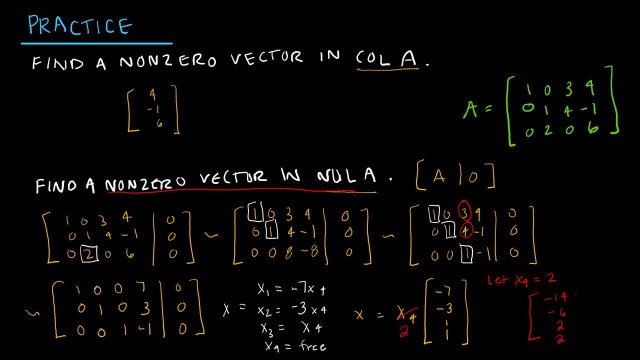 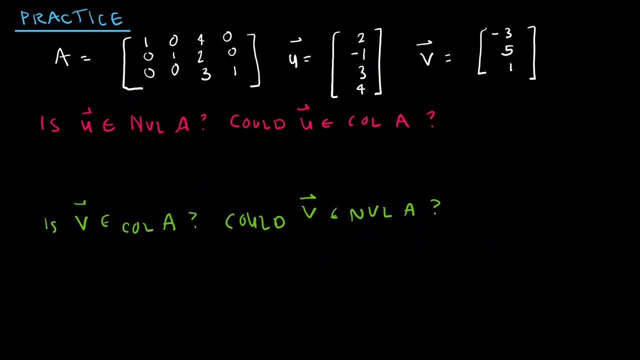 would be if I turned this into a 2,, which would give me negative 14.. Negative: 622.. So that's one of the many, many solutions. I could have a solution for any value of x4 that I chose. One last practice for us. 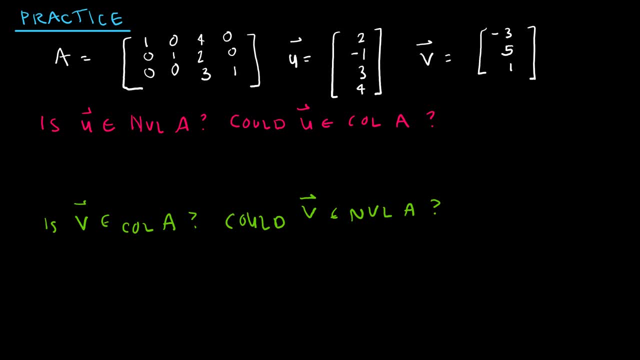 Again two parts. So press pause, press play to see how you did so. the first thing to talk about here is a with respect to you. so the first question says: is you in null a? and of course we already know how to do this. this is 1 0, 4 0 0, 1 2 0 0 0, 3, 1 times 2 negative 1. 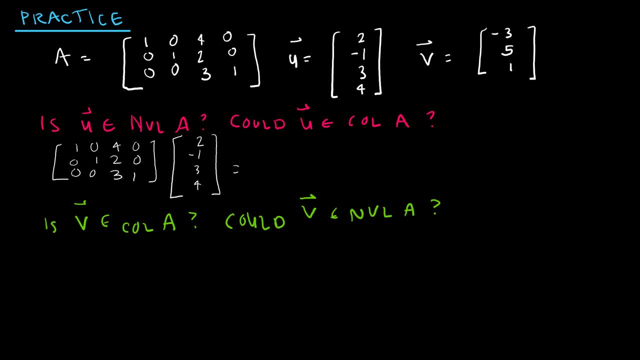 3, 4 and I'm essentially asking: is this 0? so I would get 2 plus 0 plus 12 plus 0, and do I even need to continue? because that's 14 and so this is not equal to 0? and I could continue. I would get 0 plus negative 1 plus 6 plus 0, which is 5, and 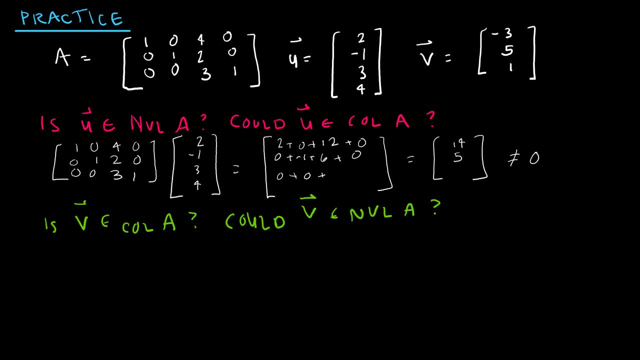 I would get 0 plus 0 plus 9 plus 4, which is 13, again not the zero vector. therefore you does not. whoops, wrong notation, you does not belong. Wow, no, a, there we go. the second part of this question says: could you the vector? you? 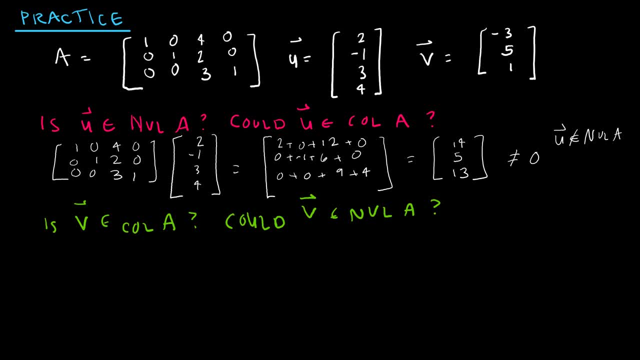 be belong to the column space of a and hopefully, hopefully. it's very clear that this answer is no, because we talked before about the column space of a. obviously that would be these vectors. so could you, which is in our for, be in the column space of a? 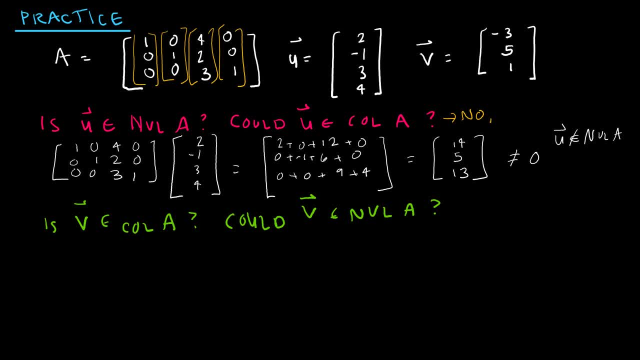 no, because column a column space of a is a subspace of r3. let me get rid of those little markings now, so let's move on to the next one is V in the column space of a. so here's a very common question. this is element Evolution videos, so what does it do here? 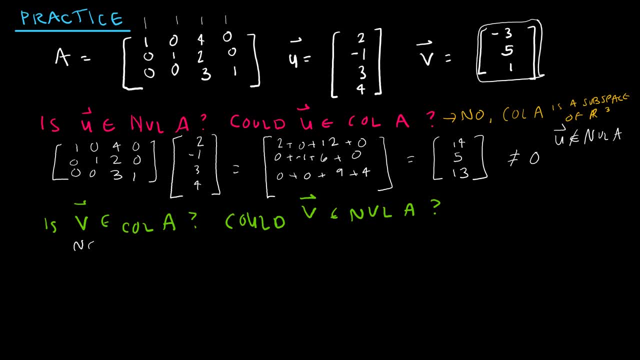 we have a vector V, so this one's node k. so, for example, let's say, if we aresel AND x and y and there is a vector column, therefore it can didn't. a no for the next characters V, V that would be K winner will still remain at aleta and a. value, let's meaning If this vector is a equally common variable, let's say value of a and c, then no in the science would be a error. and because I don't have a vector function, sure you would agree with this- the reason why we are getting along, looking here with 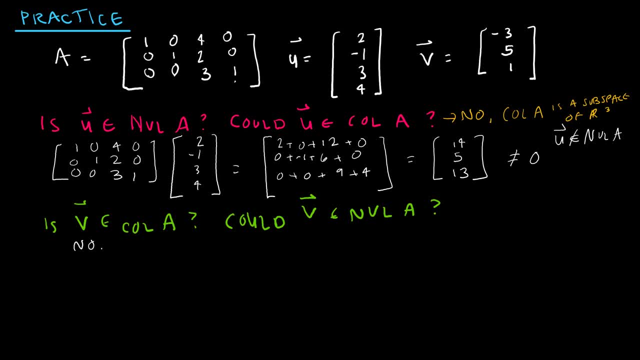 it is because, if you know that we are getting along with this, the program, this alimentos, would also be different. some wouldn't agree. I'm getting along with this, this, So good question: What do we know about the null space of A? Well, the null space of A is a subspace of R4. 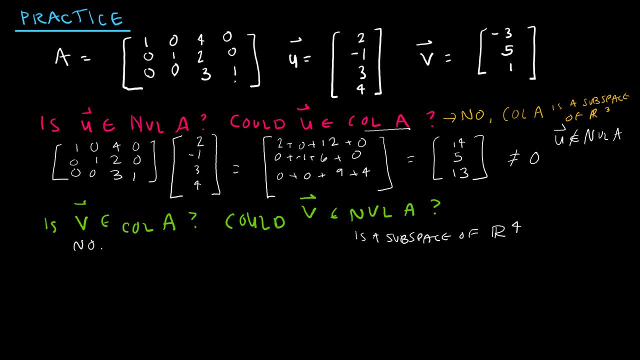 So again, the column space of A is a subspace of R3, the number of rows. The null space of A is a subspace of R4, the number of columns. So could V be in the null space of A, And again, this is a no, because it has to be a subspace of R4 and obviously V is in R3.. 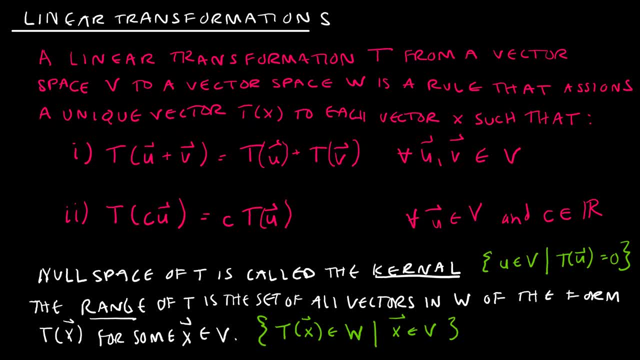 I want to sort of rewind back to something that we've talked about before and that is linear transformations. That's linear transformations, So that's not going to be our focus in this section, but it was in the textbook and I just wanted to make sure that I brought it up in the videos. 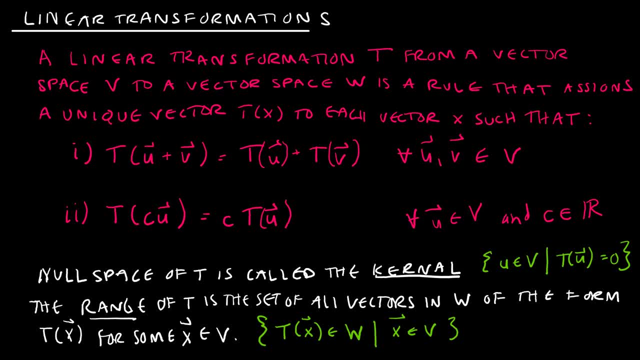 So we have talked before about a linear transformation from a vector, from a vector space V to a vector space W. Now, previously we did not talk about a vector space, but essentially what we talked about was that we had some set and that linear transformation is just a transformation onto another. 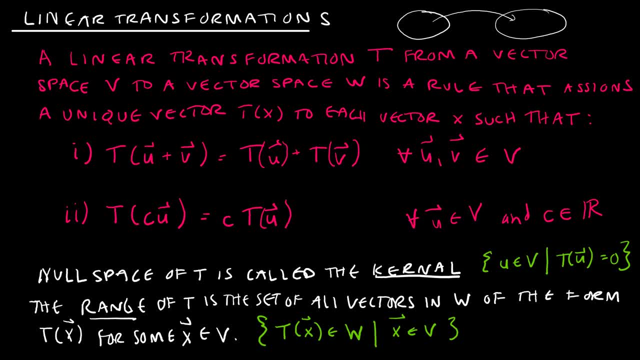 Okay, So this is a function. So, if you'll recall, a linear transformation- and again we're looking at it from a vector space to a vector space, which is not what we did previously- is a rule that assigns a unique vector TX to each vector X.